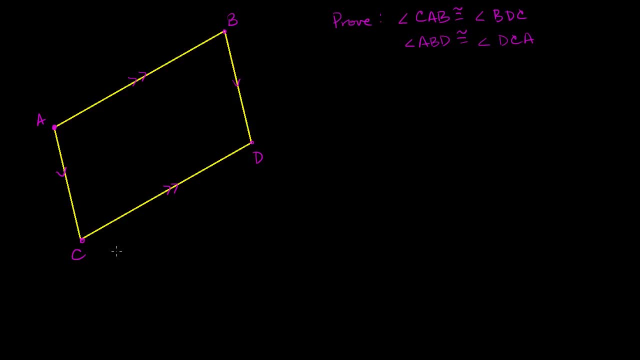 And to do that we just have to realize that we have some parallel lines and we have some transversals And the parallel lines and the transversals actually switch roles. So let's just continue these so it looks a little bit more like transversals. 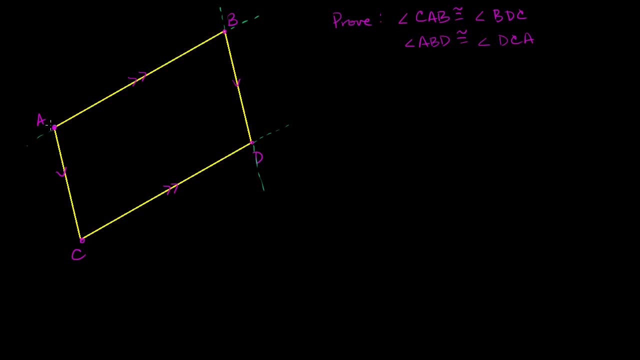 intersecting parallel lines And really you could just pause it for yourself and try to prove it, Because it really just comes out of alternate interior angles and corresponding angles of transversals intersecting parallel lines. So let's say that this angle right over here, let's make this. 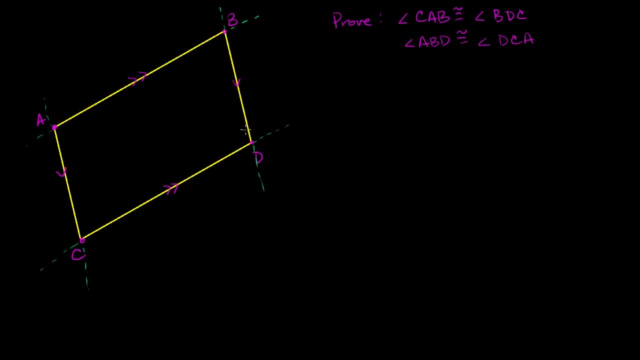 let me do it in a new color, since I've already used that yellow. So let's say, let's start right here with angle BDC. Well, angle BDC, and I'm just going to mark this up here: Angle BDC. 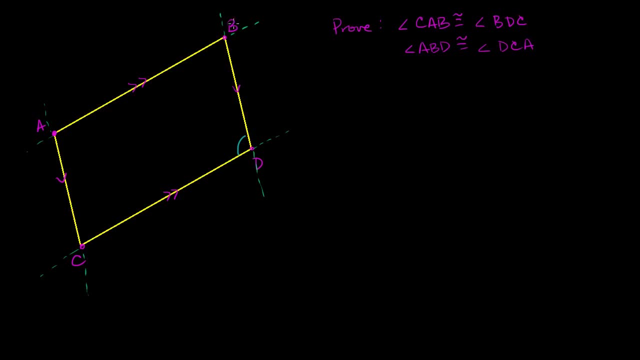 Angle BDC right over here. It is an alternate interior angle with this angle right over here, With that angle right over there, And actually we could extend this point over here. I could call this point, I could call that point E if I want. 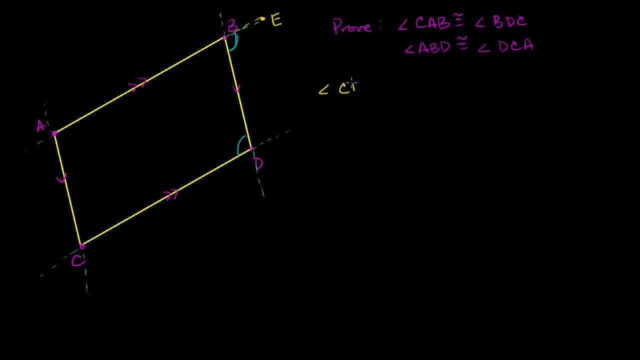 So I could say: angle CDB is congruent to angle EBD, Angle EBD by alternate interior angles. This is a transversal. These two lines are parallel. AB or AE is parallel to CD. Fair enough Now if we kind of change our thinking a little bit. 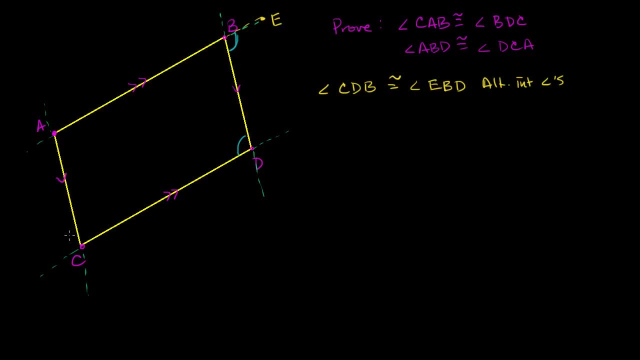 and instead we now view BD and AC as the parallel lines and now view AB as the transversal, then we see that angle EBD is going to be congruent to angle BAC Because they are corresponding angles. They are corresponding angles. 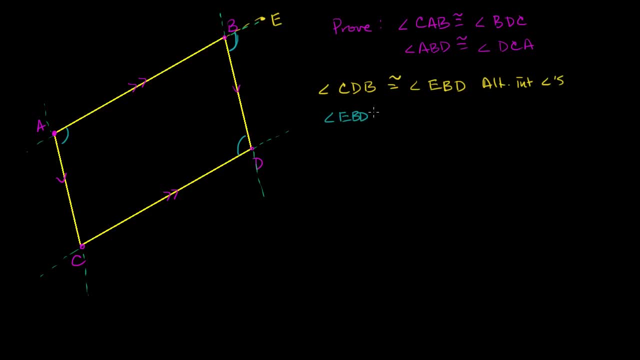 So angle EBD is going to be congruent to angle BAC, Or I could say CAB, Angle, CAB. They are corresponding angles And so if this angle is congruent to that angle and that angle is congruent to that angle, 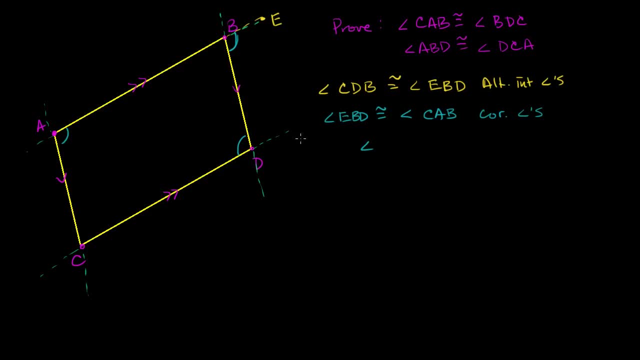 then they are congruent to each other. So angle C- Let me make sure I get this right- CDB, Or we could say BDC, is congruent to angle CAB. So we've proven this first part right over here. And then to prove that these two are congruent,